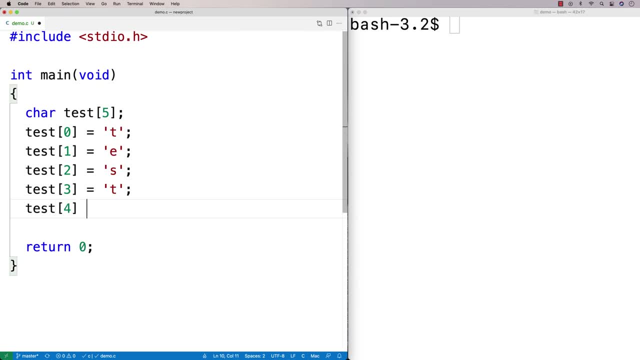 my last character in the string I'm going to say test 4 is equal to this special character here: slash 0,, which is the null terminator. Then I'm going to say printf and I'm going to say percent s to print out the string. I'm going to do slash n, then I'm going to say test here. 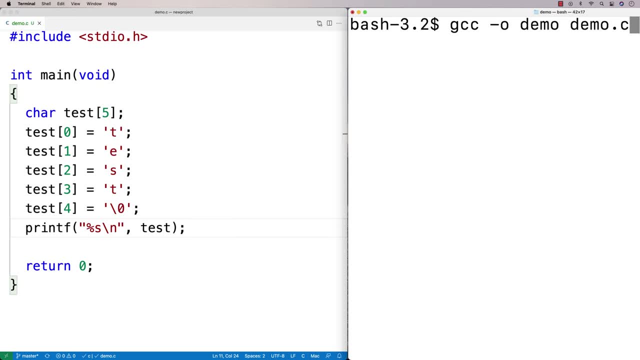 Now, if I go to print this out, we'll see that test is going to print out. We're not going to see that null terminator though, because that's actually a special character. It's actually a non-printable character and it just terminates the string. 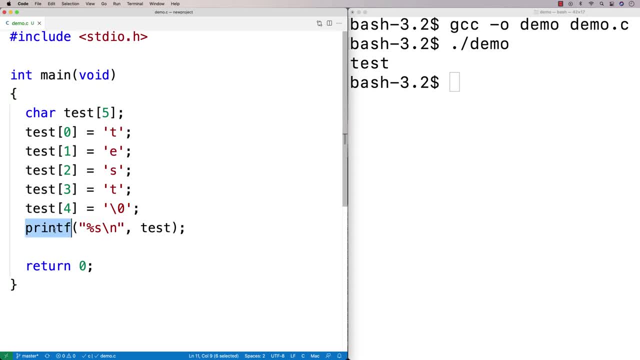 It just signifies the end of the string. So when we use printf here and we give it percent s as a placeholder, we're telling it we want to print a string And then we give it the string here, test to print. And that's how printf knows that the 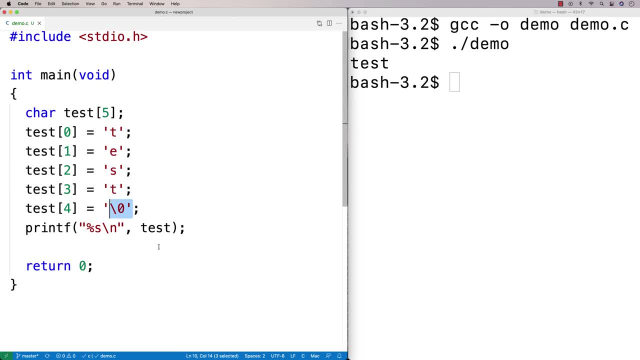 string is done, is this null terminator there that ends the string. Now we don't have to actually set a string with each of these. We don't have to set a string with each of these, Each individual character, like this. There's other ways of setting a string in terms of: 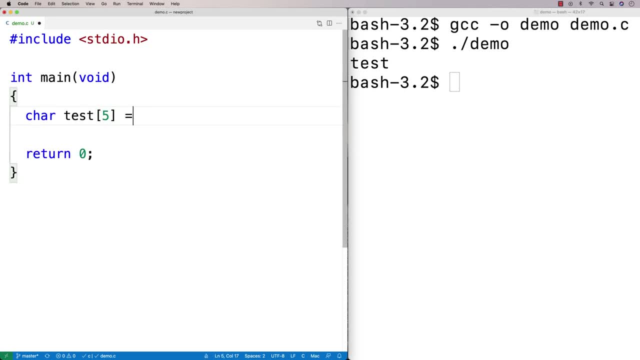 initializing it with some initial value. So I could set it like this too: I could say: test5 is equal to test, And then, same thing, I could still printf test and print it out. And what's going on here is this is what's called a string literal, And when C uses this string literal here, 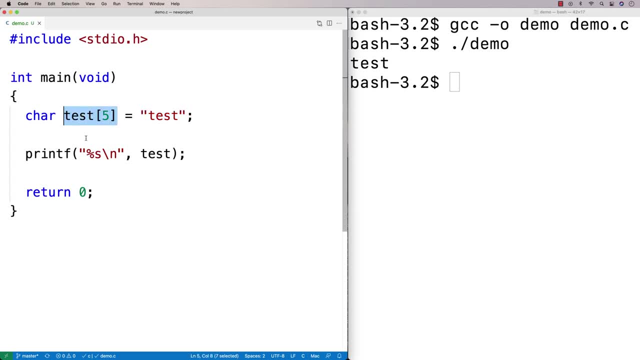 to initialize this test array here. it knows that we're initializing it here to a string, So it's going to automatically put in that null terminator for us, And so I could run this here And we'll get test out again, And I could also do things like create a loop to access each individual character in my string. 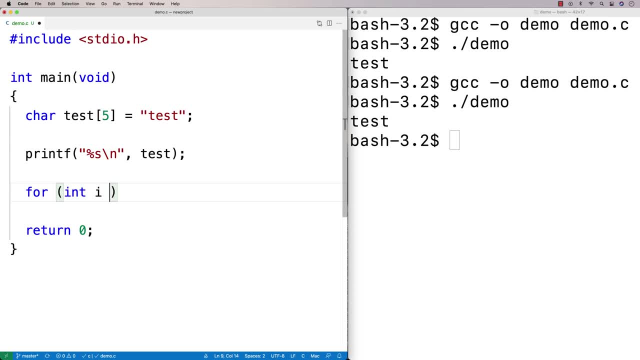 too. So I could say here: like 4 int, i is equal to 0.. i is less than We'll say 4 here or 5 here. We'll say i++. And then we'll say here printf, And we'll say percent c And I'll say test. 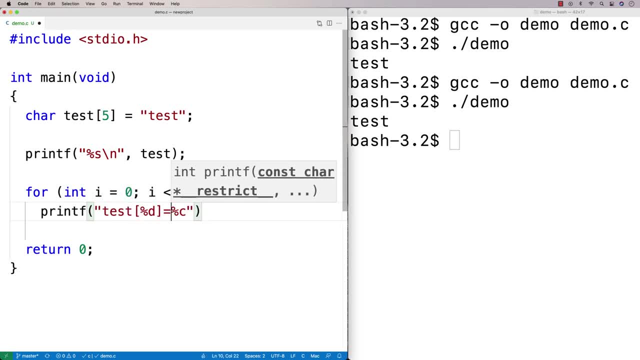 At percent d is equal to percent c, And what I'm going to do is I'm going to print out i and test that i And we're just going to be able to see each individual character of test here, And I'll actually just put some single brackets around the percent c there. 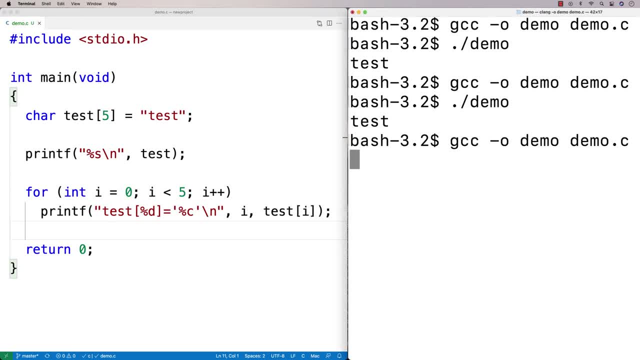 So what's going to happen here is we're going to find that the null terminator isn't actually printed out. So we get like test0 is t, test1 is e, test2 is s, test3 is t, But then this last character here, the null terminator. 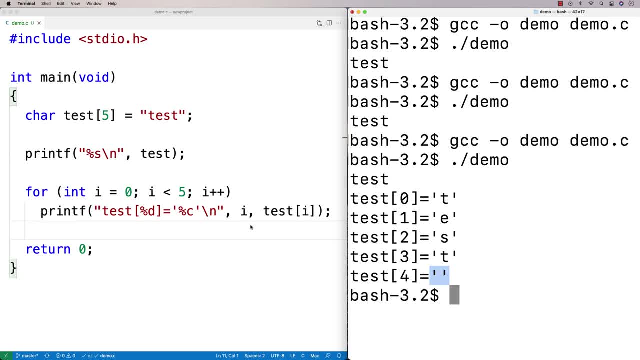 we get nothing. And it's just because it's a non-printable character. It's not something that's actually for printing out. We don't have to use a number here when we initialize strings either. So I could say something like this. I could say: like car test2 is equal to, And I could say some big 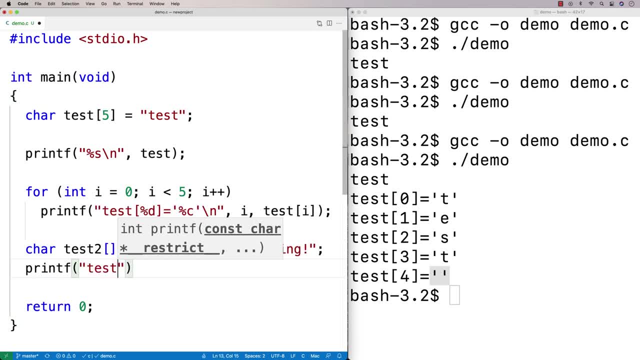 long string And we could print this out as well. And this is OK. We can do this. C can figure out how big of an array to make test2 based on the length of this string literal, And so we can run code like this: And this is OK, And so we'll get test2, some big, long string. 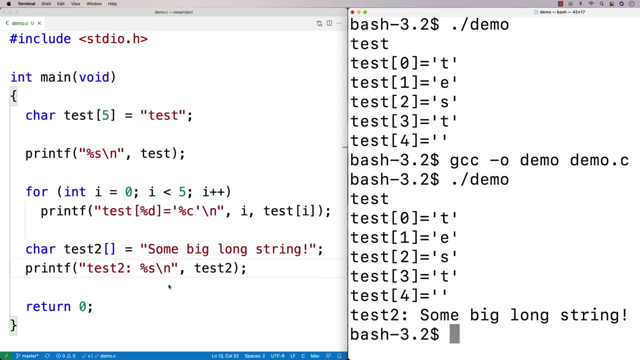 So now, one important thing when working with strings is the string library, And I'm going to make a separate tutorial video covering just the library, because it's got a number of functions in it. But what I'm going to do is I'll go over a couple of key ones. So we're going to say number. 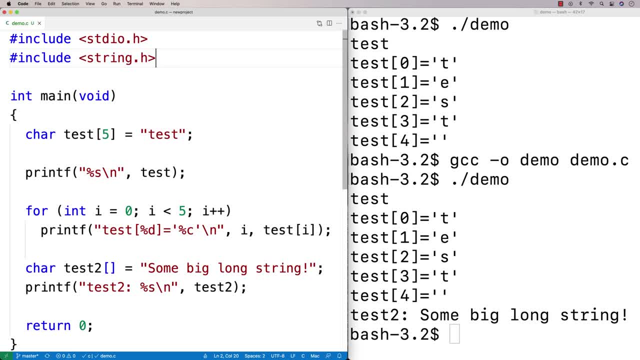 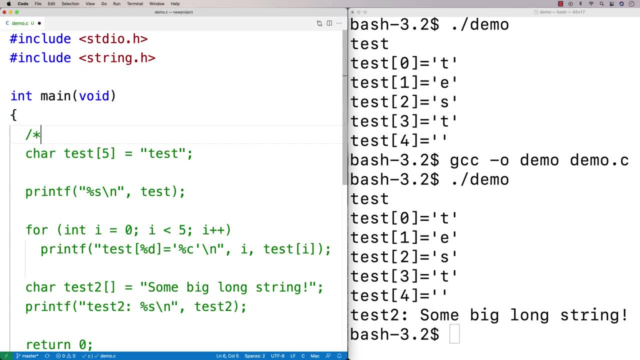 sign include And we're going to say stringh And what this has is functions that allow us to work with strings in a string library. So we're going to say stringh And we're going to say a nice way. So I'm going to say that I'm going to comment out this code And I'm going to use some. 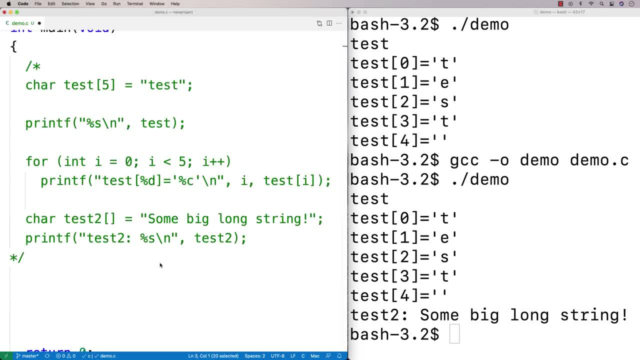 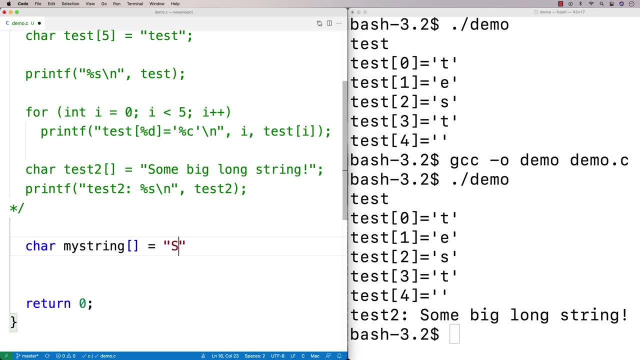 of the functions in this library here to work with strings. So one of those functions is called string length And the way it works is like this: If I have some string, I'll say here, car my string is equal to some string. exclamation mark, exclamation mark, exclamation mark. And I'm 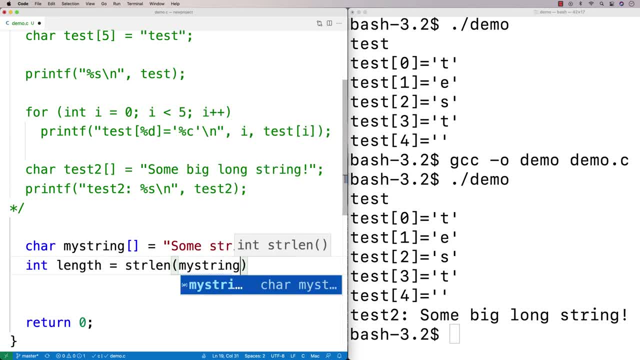 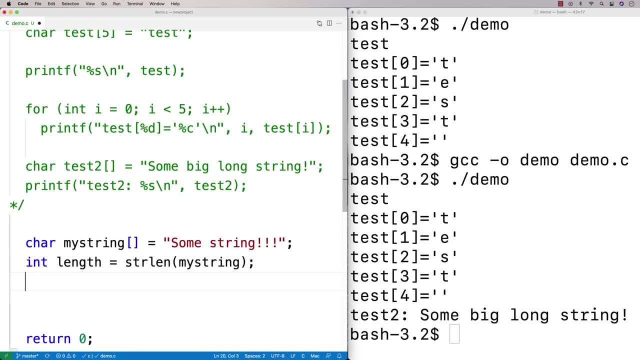 going to say here: int length is equal to string length of my string. And what this will give me here, this strlen, it's going to give me the length of the string And we'll just print it out. We'll say printf And we'll say length, percent d slash n And we'll 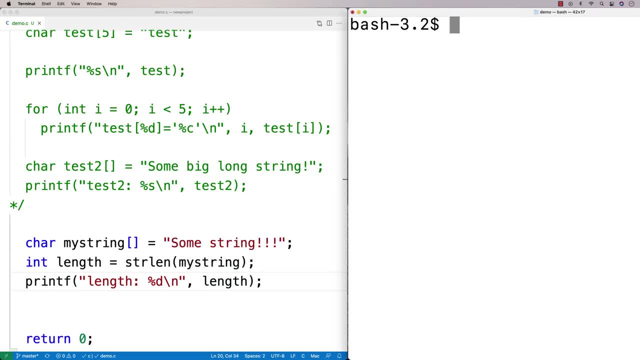 output the length And let's just see what we get here. So I'll clear this. I'll run a compiler here, I'll run the program And I get length of 14.. So let's actually see what length is actually giving us here. So length is actually giving us here: 1, 2, 3, 4, 5, 6,, 7,, 8,, 9,, 10,, 11,, 12,, 13,. 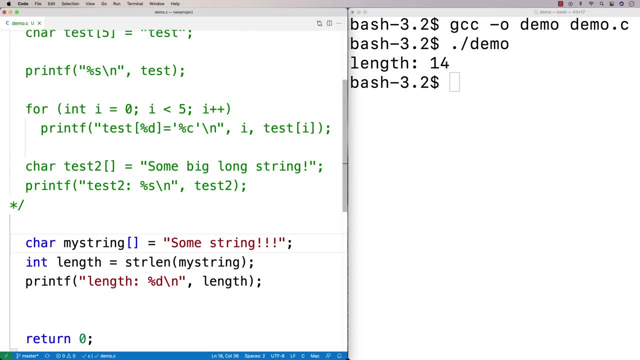 14.. So length gives us the length of the string, not including the null terminator. So just remember that The null terminator is not included in the length of the string, which makes sense because the null terminator, as much as that's part of the string in the sense that it's a special. 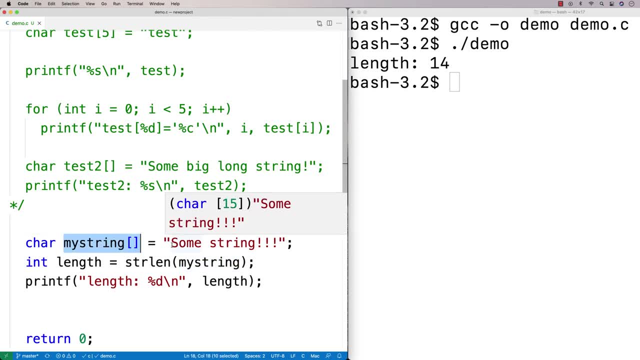 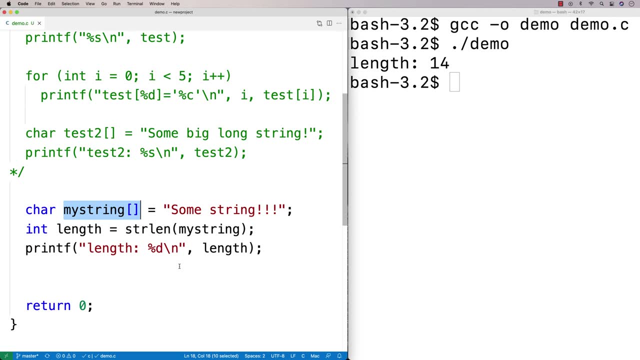 character. it's not really the length of, it's not really part of the length of the string that we care about, right? So if I wanted to do some work with my string, for example, like maybe I want to count the number of, maybe, let's say, S's that appear in the string, I could do a loop. 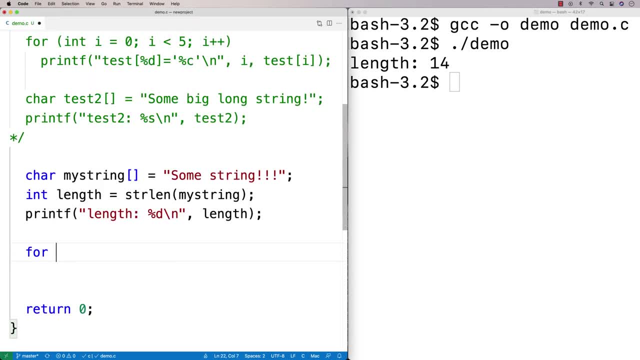 that uses string like to help me do that. So I could say here: like 4 int, i is equal to 0, i is less than length, i plus, plus, And now I'm going to have some code in here that's going to count the. 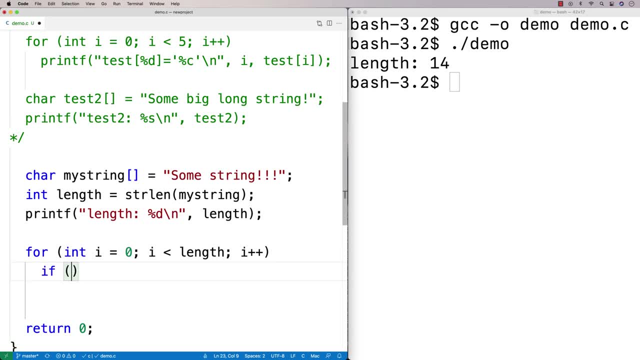 number of Ss. So I'm going to say here: if my string at i is equal to S, or my string at I is equal to S, capital S, let's increment the length, the count of s's, and i'll have to make a variable to count that. so i'll have to say like int: 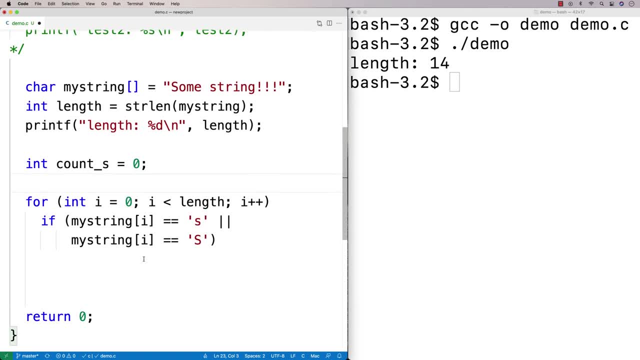 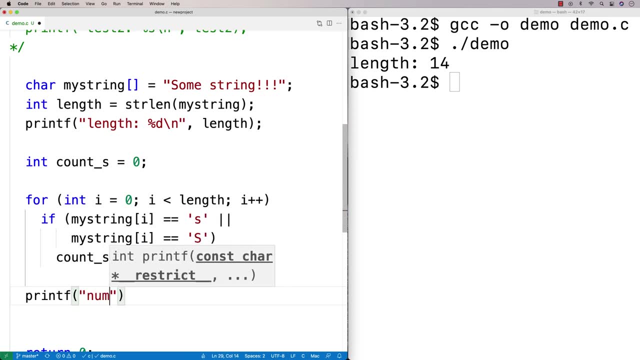 count s is equal to zero, and then i will increment the count of s's here, so i'll say count s plus plus, and then i could print f, the number of s's, so i'll say like number of s's, or maybe i'll just say: count the s, count percent d will output the, the count of s's, and 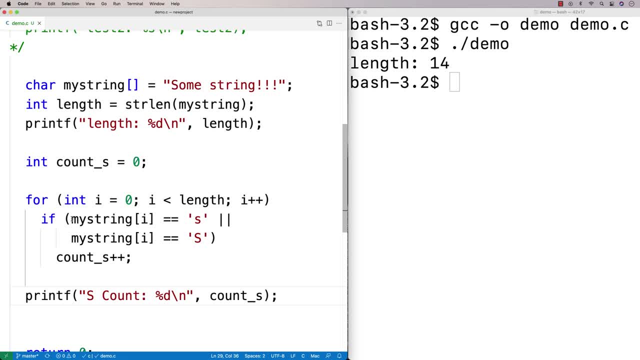 what i've got, what i've got here now is i've got code that's looking at every character in my string up until the length of the string and i'm checking to see if that character in the string is s lowercase or s uppercase, then increment the count of s's here. so if i run this here,